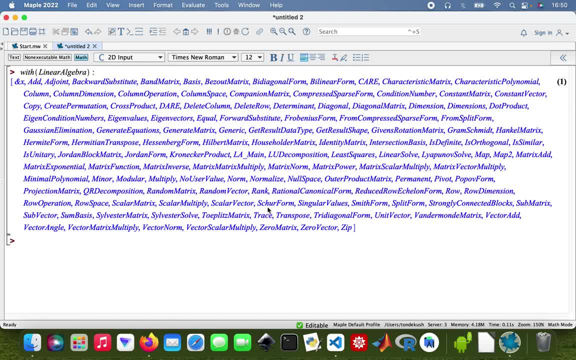 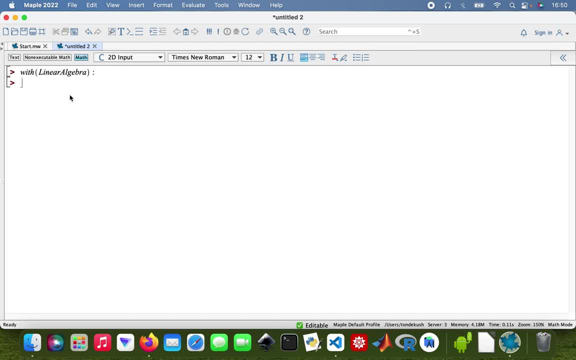 You can type in a colon as well. So if you don't want to show all this information, just press the colon. type in the colon. Okay, cool, So I've got my system, so I'll call it sys and a square bracket. 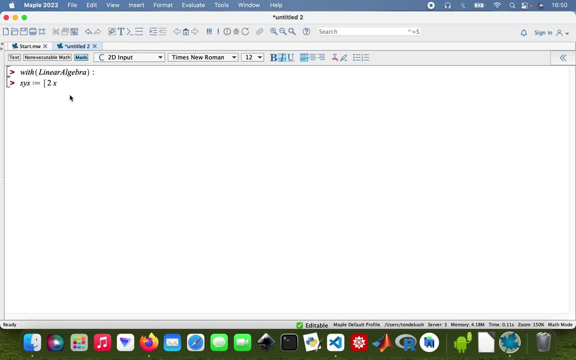 So 2x. So I'm going to use subscript. So command shift and then underscore, That's 1.. Okay, and then the next will be 4x, then subscript 2.. And then plus 9x, subscript 3.. And then 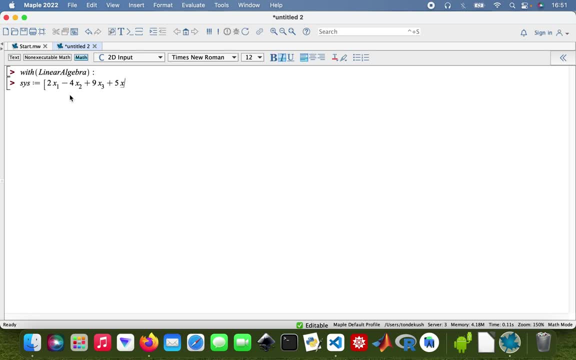 that's sorry. plus 5, 5x and then subscript 4.. So that's equal to, that is equal to 1.. And then my next equation: so we'll be following the same format, x, And then command shift and underscore, And that will give you the subscript option. 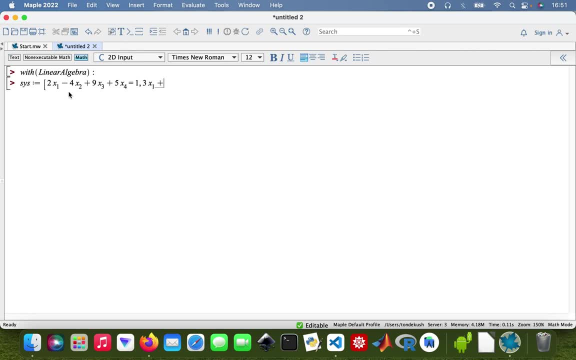 So that's: 1. Yeah, plus x subscript, 2. Plus x subscript, 3.. And then minus x subscript, 4. Yeah, so that's equal to 6.. Alright, and then I'm just going to create an array, a vector, with my variables. 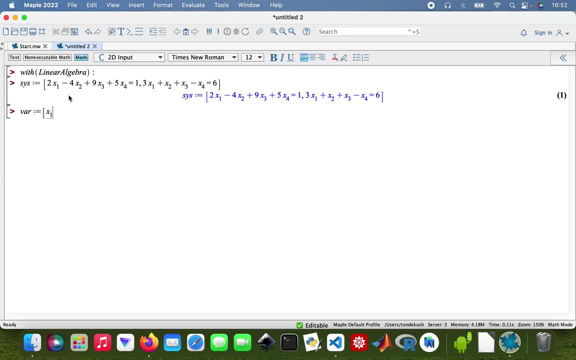 So x, subscript 1.. And then, sorry, And then x, subscript 2.. Right, There we are. So those are the variables, Right, so I'm going to generate a matrix Of the matrix itself, or the system equations and the vector with the variables. 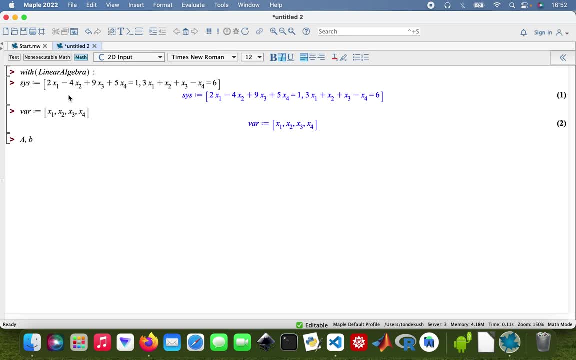 so I'll type in this: a AB and that's equal to you. generate matrix and system and involve. okay, yeah, I'm just gonna multiply out, so, times the vector, that's equal to B, right, and then what I need to do now is I need to create an augmented 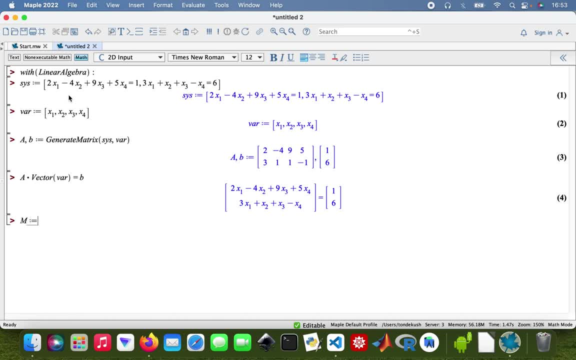 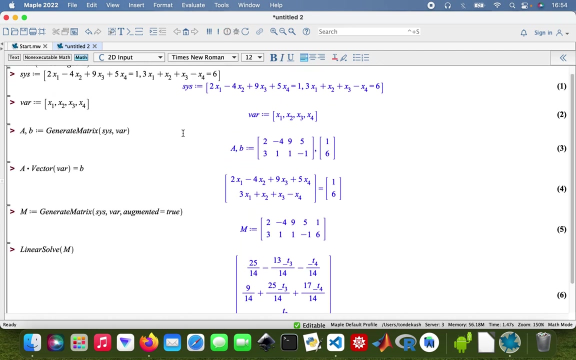 matrix, so M equals. so generate matrix again, system. and then here are not, here are in football, haha. then augmented it matrix that's equals to true, so yeah, so now I need to solve it. so then you solve matrix M and voila, there we are. I can also do another one just using using my variables, as, sorry, I'll. 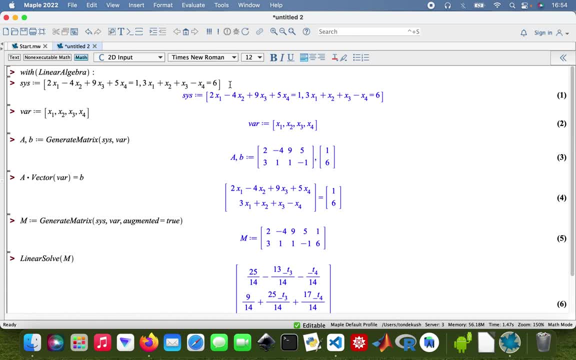 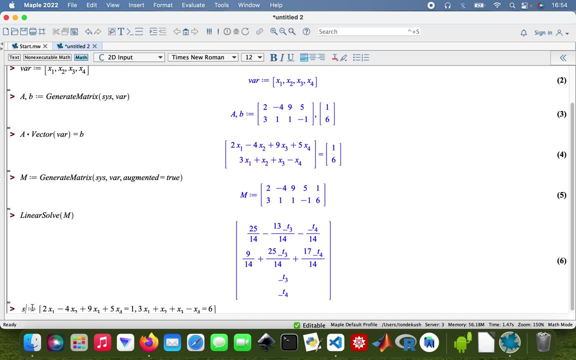 change. I'll change the digits, I'll put zero there and a zero there, so the same thing. so command, copy and then paste, but I'll call it equation, okay, and then I'll use the same variables as well, okay, so what I'll do is I'll just do a linear solve. 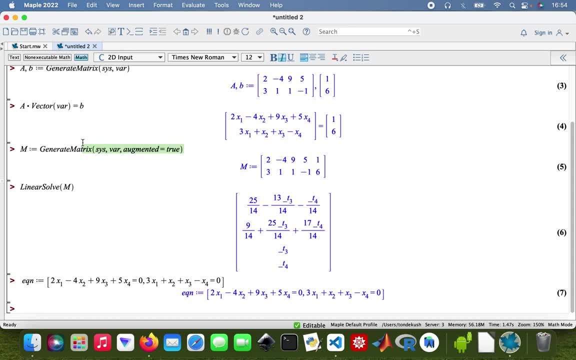 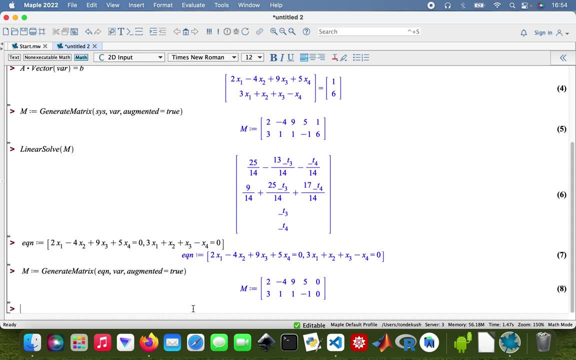 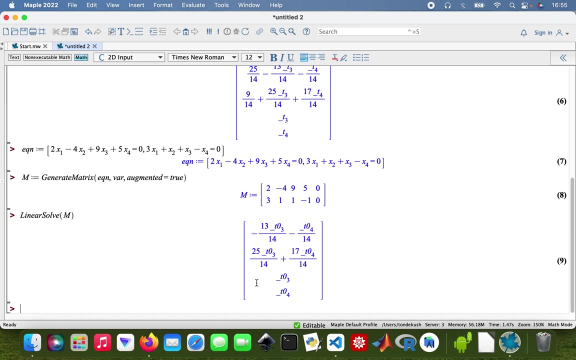 you. here's my formula for the absolute data. let's do that. so all right, okay. so the answer I need myself, so do this, all right, okay. so now it's the basic definition. so I'm going to support my copy this, that there, and then that's the other. so all speech factor. so I'm only 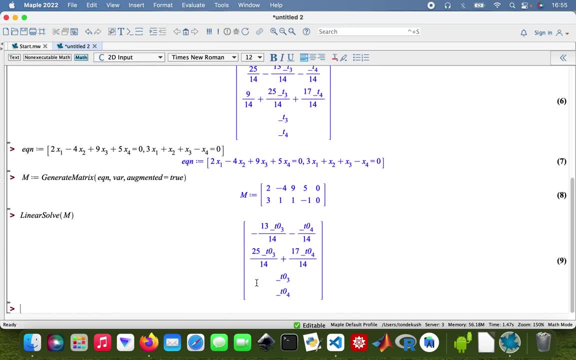 doing this to moderate all that. these functions. here it comes down to min muli, cool. so it's just a quick read on how to do a linear solve in maple and just to solve a system of equations, okay, cool. so thanks guys for watching, and I have a.